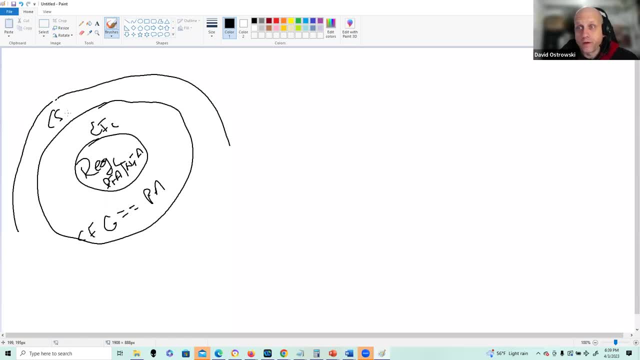 to be context-free, okay. Or, specifically, instead of having some self-defining terms that you typically see in most textbooks, how does this compare? okay, to something that isn't context-free, okay? Well, the next step up in complexity might be: would be considered: 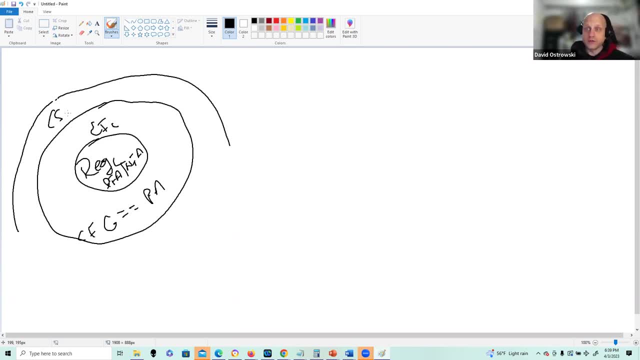 context-sensitive. Our classical examples of that could include capitalization of a first word, the first letter of a first word in a sentence- The cat ran to the hill, So I have the represented twice- and setting up the rule for capitalization. what's the difference between? 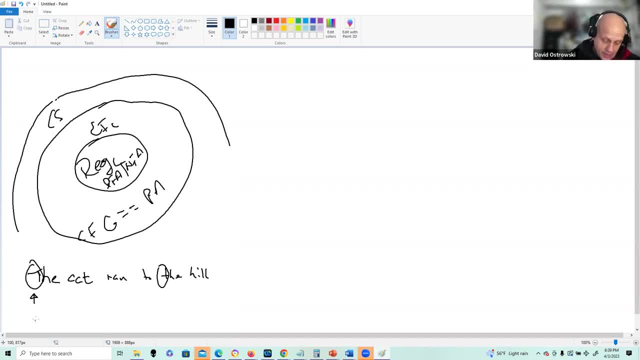 each of the words Where- well, in this case, it is the I have to take. I have to be sensitive to the context in which I've been using it. If it's the first letter in the word, I'm going to capitalize it. If it's not, then I'm. 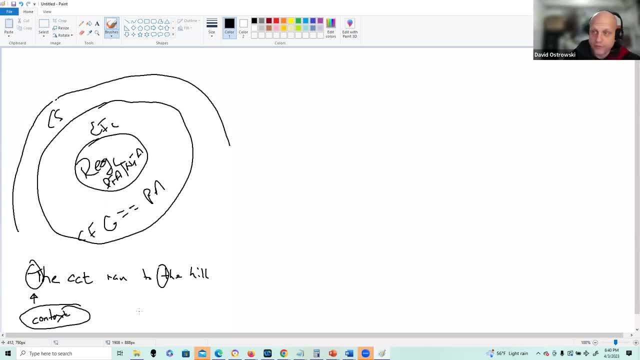 not going to capitalize it right: Similar nature. let's say I before E, except after C. right Rule in English spelling Let's say say receive, and it would be E-I as opposed to I-E. Okay, 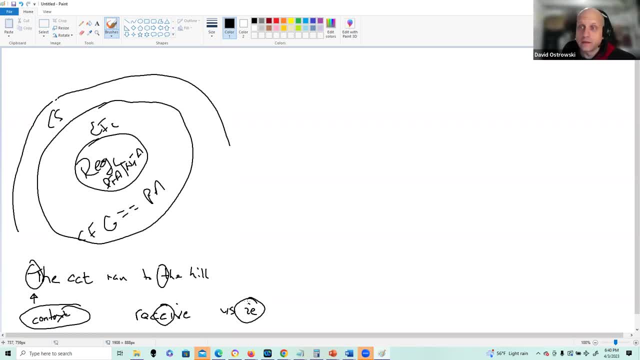 What's the difference? Well, it's whatever following the letter C. So we see a couple of things: dynamics here, or similarities between regular and non-regular. is the fact that I have to remember something, I have to use extra memory. In this case, I have to use extra rules. 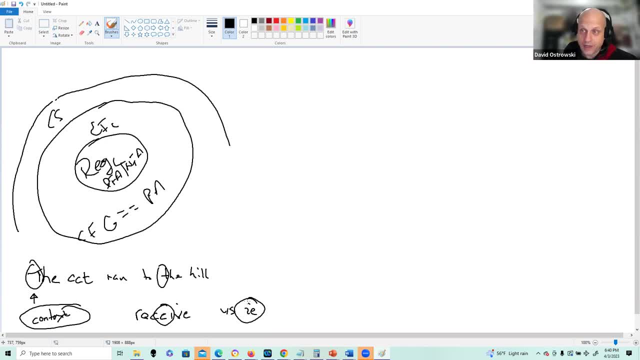 and perhaps even more memory. Okay, Then, what I would use to define context-free- So another layman's term, the context-free, uh grammars- would be general grammars. Okay, Very, very, our most basic grammars. 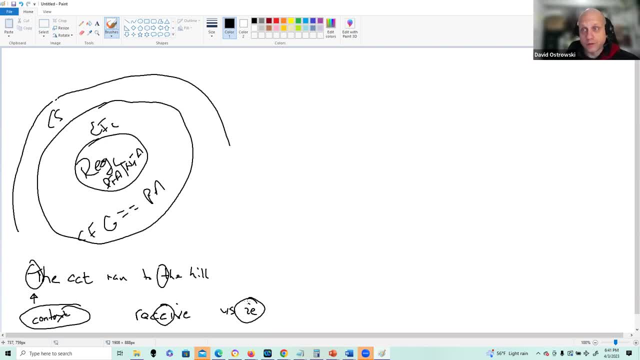 which are defined by a non-terminal on the left-hand side of the assignment and terminals, or non combination of terminals, on the right. Okay, And we increase in both complexity and the amount of memory that's being leveraged as we expand our categories to- uh, even to the level of 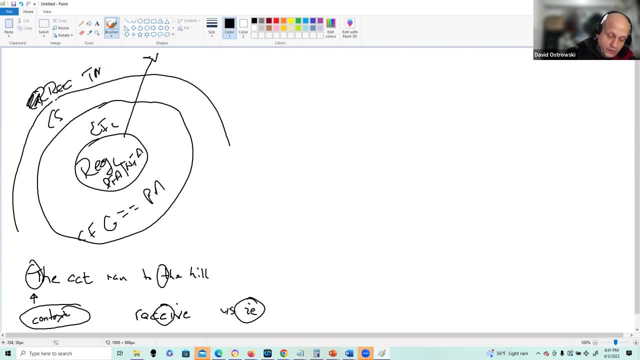 uh recursively enumerative. that would require a Turing machine, which is? you had another uh more expansive uh operation and could it be expressed in terms of states, just like with DFA, NFA, pushdown automaton, except in this case you have a. 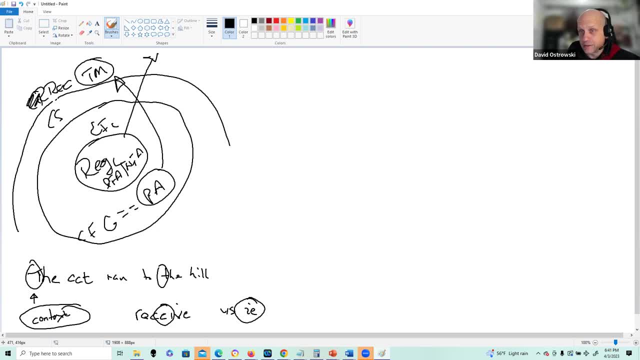 complete fully operational link list, if you will, Okay, Or uh tape where I can move forward and backward and use multiple dimensions as well. So, um, so that's the direction we're going to. that puts everything in context of where we stand. 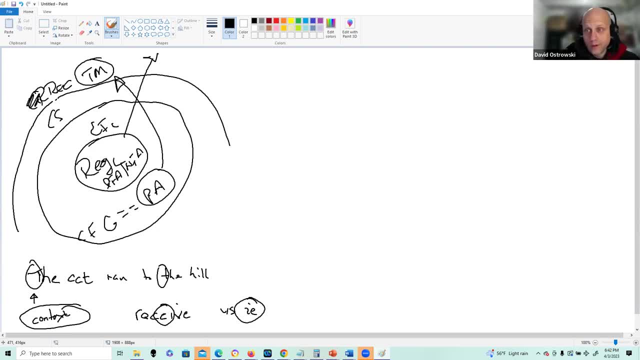 and sets us up for a little more, uh, well-informed, uh, definition of what we're referring to when we describe pushdown automatons, Right, So, uh. so let's look at one of our classic problems for context-free grammar And, in this case, instead of using a grammar to solve it, 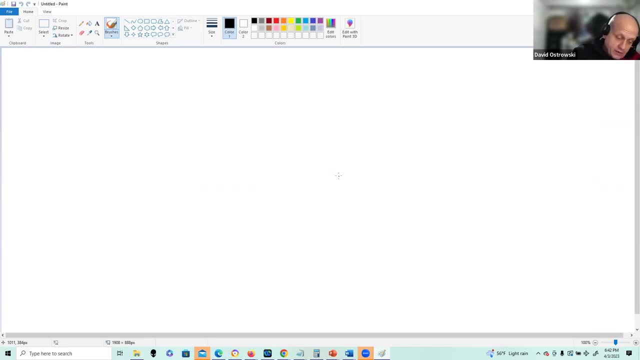 I'm going to use a pushdown automaton. Right, And here again, our regular language was A-N-B-M, over the language of all A's and B's. Uh, but A-N-B-N is non-regular and requires a grammar to solve, as opposed to a regular. 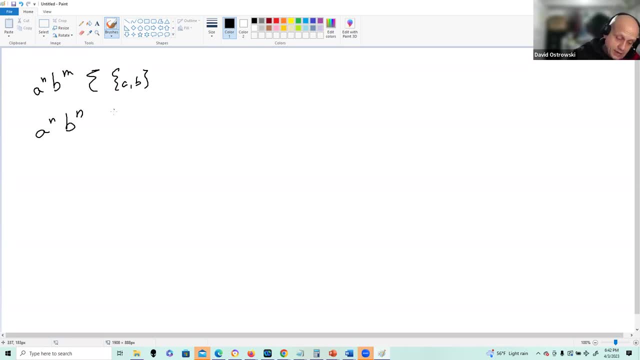 expression, or FA, DFA, And I can use a PDA pushdown automaton, uh, to solve this. Why? Because it allows me the same transitions, for the exception that it provides the means of operating to a stack. Okay, So if I look at, 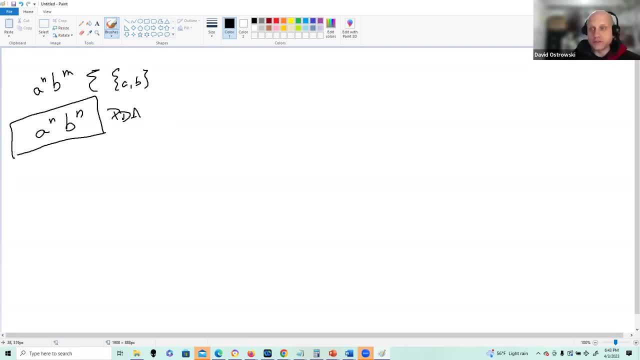 and I try to think about what's the, the, the simplest structure that I might need to solve this problem programmatically. if I'm looking at a language of all A's followed by equal number of B's, say A-B-A-A-B-B-A-A-A-B-B-B, so on and so forth. 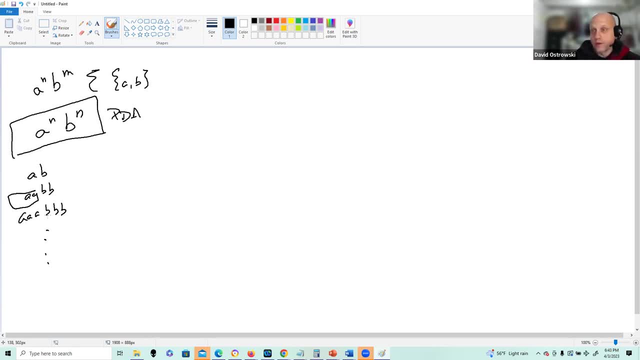 progressing on, I need to count uh the number, or I can push and pop From a stack, So I can think about this in terms of an automaton uh. for the exception, I have to put in an uh extra operation and that is operating to our external data structure. 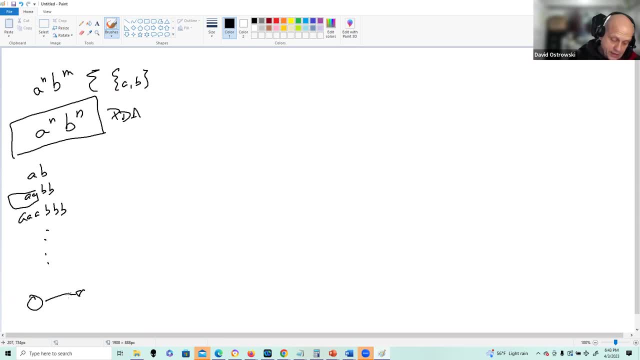 So I can look at this as this problem, as uh, uh, a starting structure where I'm going to uh, continue the loop, And from an English language I can say, uh, I would be pushing to the stack that this is in the case of all the A's, And then I'm going to make a transition. 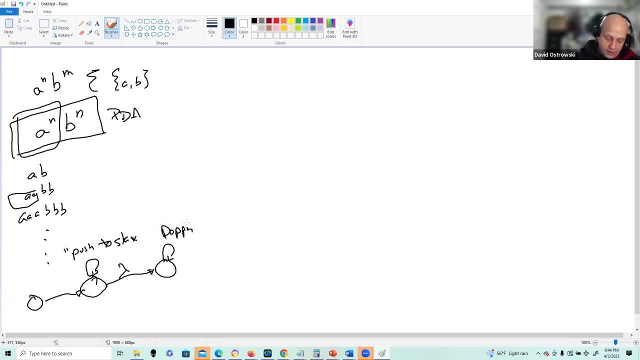 to where I'm going to be popping from the stack. Okay, Uh, and I don't have to transition on lambda transition on the first B in this case. if I were just examining a count, then I would need a lambda transition, um, but it'd be popping from the stack And what's going to put me in a final state is my 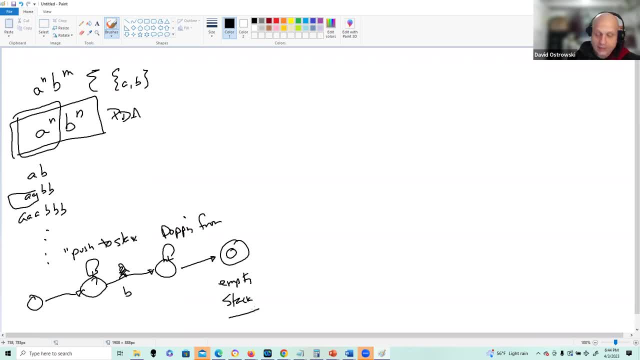 empty stack. Okay, So that's from a language- English language based description how I would exactly solve this problem, Right? So let me write down the solution. We'll work through it and clean it up a little bit, Okay, And give you complete, uh explanation. So the alphabet, the final states, the initial states. 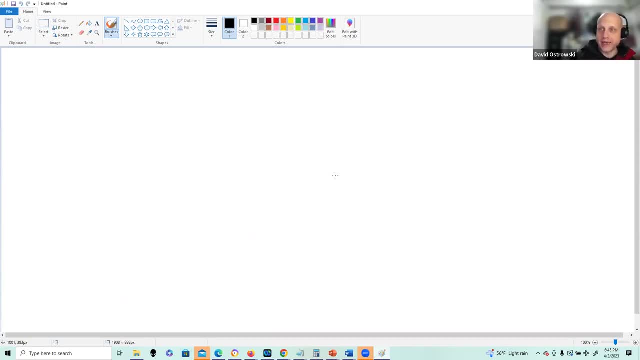 our formalized definition is all the same. Let's just look at it, The basic mechanics, and have the general understanding that here, when I'm looking at the context-free grammar, it's all about the support of that transition and the operations on the uh pushing to the stack right- So great. 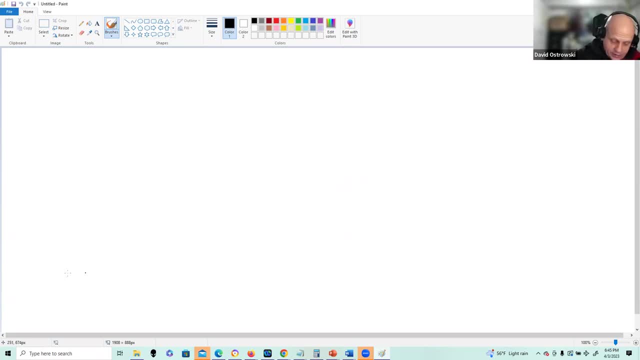 So let's look at the transitions and I can look from my starting state. here I have a state of 0 And I can go to a state of one And again that is my I'm going to push And the state two, so I'm going to pop. 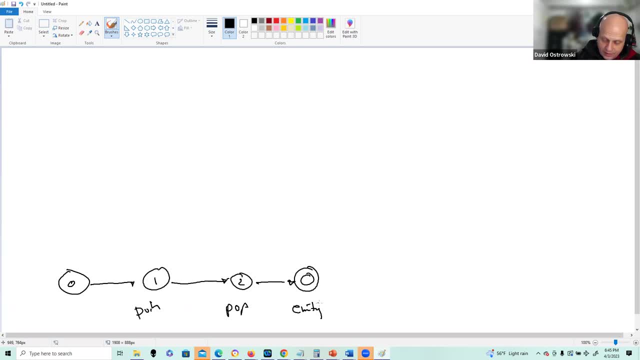 And then, hopefully, if I have an empty stack, I'm going to transition to final state. If I don't, then I'm going to end up remaining in the state two in most cases right. So that's how it's going to look from an FA type perspective or a dominant perspective. 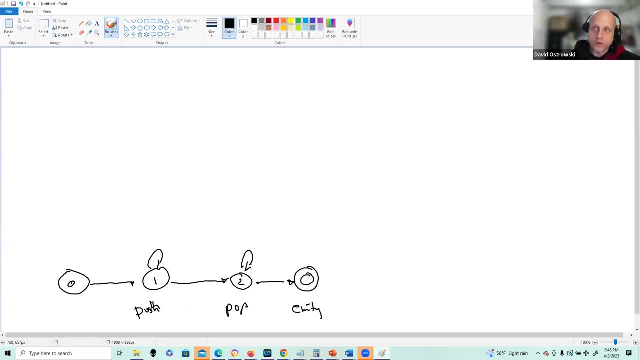 I won't say finite and dominant, because it isn't finite right. It is a little more powerful than that, right. So here I'm just going to outline my transitions and I'm going to write the state here And sometimes use an alphabet to. 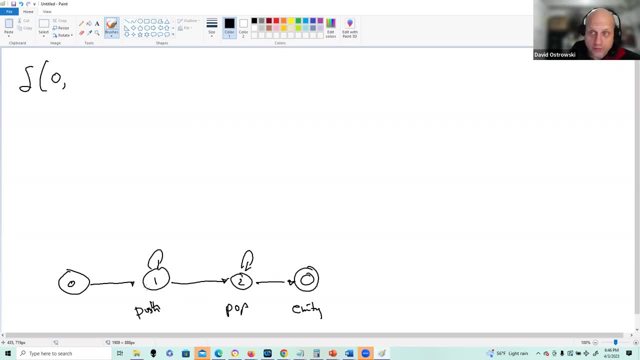 Work with the stack to differentiate between input alphabet and alphabet, that I'm operating the stack here. I could just push and pop. I don't have to worry about that too much, right As long as I keep them straight. So in this case I can. I can say: 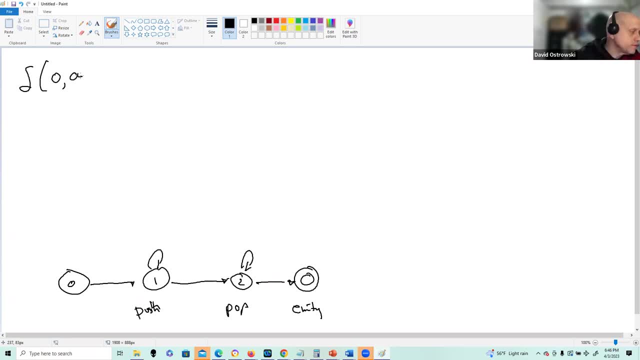 A as input And I can use a. Z Can be The equivalence of an empty stack, right? So I can put Z down here, just to remind myself, right, If I will? And in this case I can make the initial transition to. 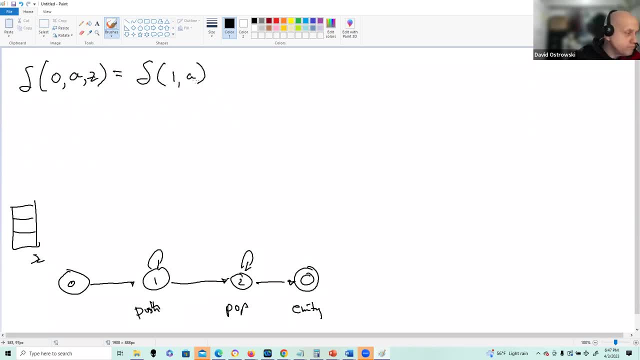 State one, And this case I'm going to push that A to the stack. So in typical operations I'm going to pop here And I'm going to Push. in most cases, when I'm doing the pushing to the stack, I'm going to be not only pushing my input character but the character that I pop from the stack. in this case I don't pop anything. 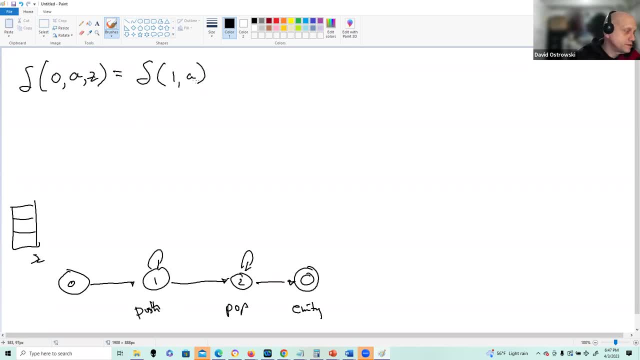 So I'm not going to push anything more than that single letter right. So that's my single transition that I have. I could have Nondeterministic NFA right, And I could say OK on a state zero. let's say I have an empty stack and and Z, then I just skip to the state three. 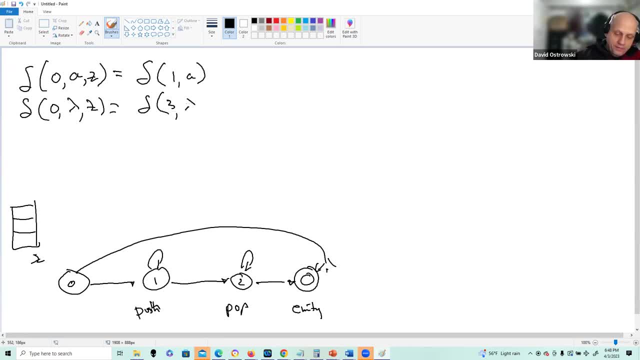 Right And and push Lambda and that would give me the solution Right, Empty alphabet. OK, so the null character, if you will, It could fit in my alphabet right. So We covered this in our FA. let's move forward. so here I'm, operating from the, the first state. 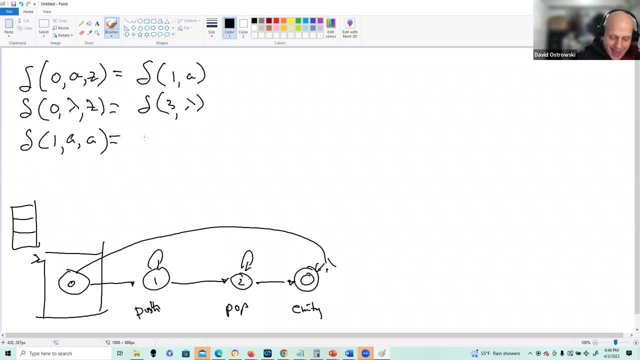 And here I have an input alphabet character A, and, and I pop from the stack. let's say I have an A because I already pushed one to the stack, Then I'm going To transition in that loop and I'm going to, in this case, push A to the stack. 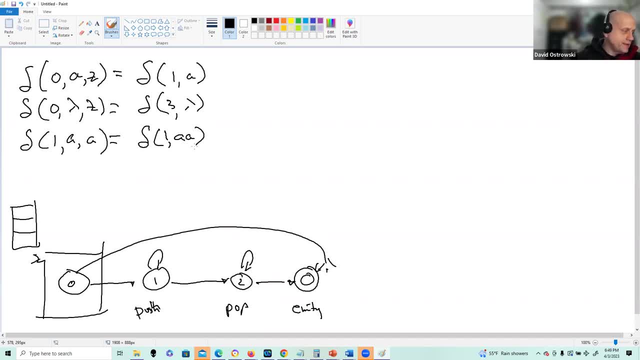 Right, And, and I can keep on going like that: Right, And, and, and that is really All the operations that that I'm going to have. right, So that addresses all of The transitions from State one, for the exception of B, right, so if I have one and I have a B and I popped an A, then I would go to state two and I would be. 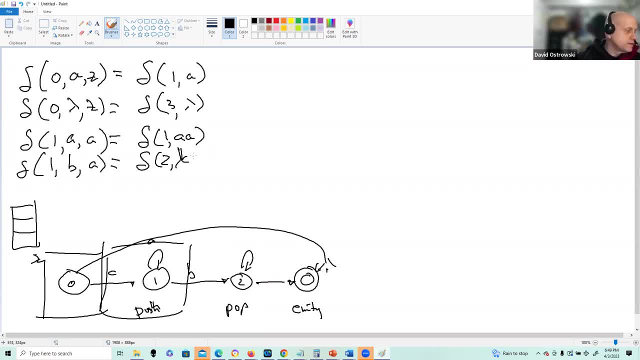 Popping from the stack right And correspondingly I would continually be doing that operation. I would take a transition from state two. In this case I have a B and an A as input. then I would transition back to the same operation here. 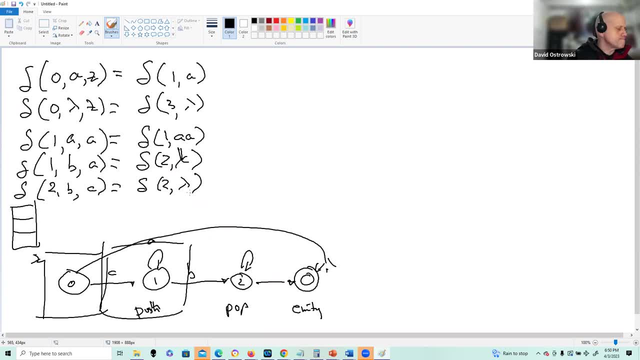 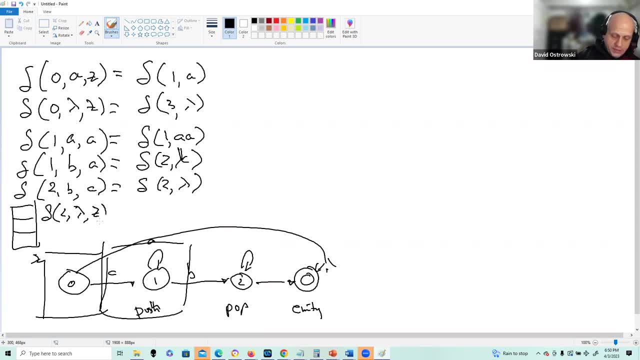 In that case I would check for Z, OK, and if I have Z, then I would transition to C3 with the Lambda and then I would be done. This, essentially, is telling me I have the empty state. So So these two are from actually from this operation here, and the pop operation is. 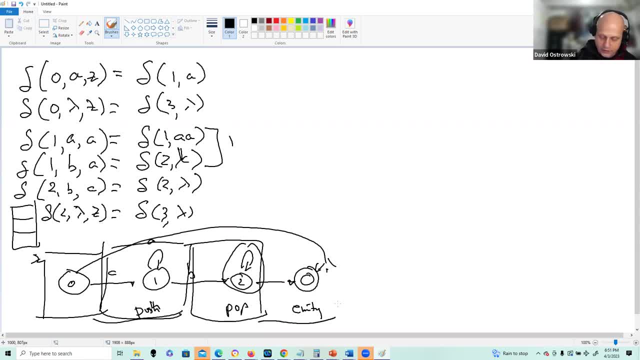 Managed here. that's this loop, And then from here I transition to the final state, given that I have the, the final solution. So let's just try this really quick with one of our examples. I have a, A, B, B.